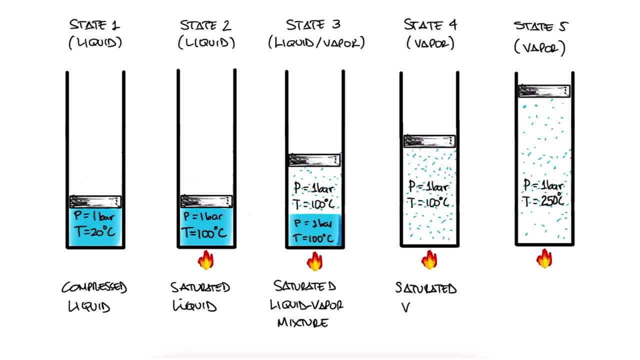 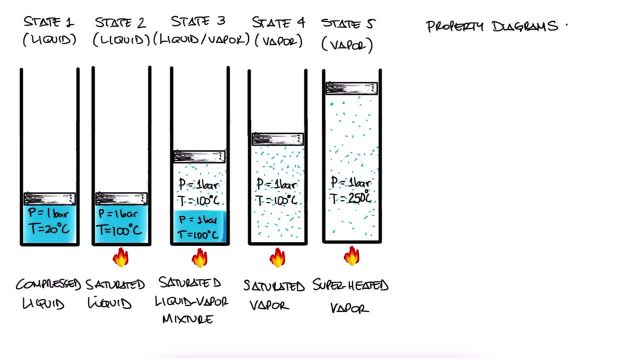 saturated liquid vapor mixture, saturated vapor and superheated vapor. In thermodynamics we'll constantly use property diagrams to show the states of our system and the processes they undergo to go from one state to the next. One of the most common 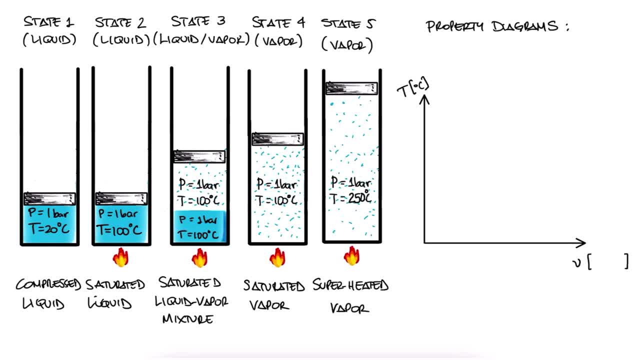 ones is temperature versus specific volume. If we plot these five states in a TV diagram, we'd see 20 degrees Celsius on the y-axis and roughly 1 cubic centimeter per gram on the x-axis for state 1, then up slightly, moving right as the density decreases. when 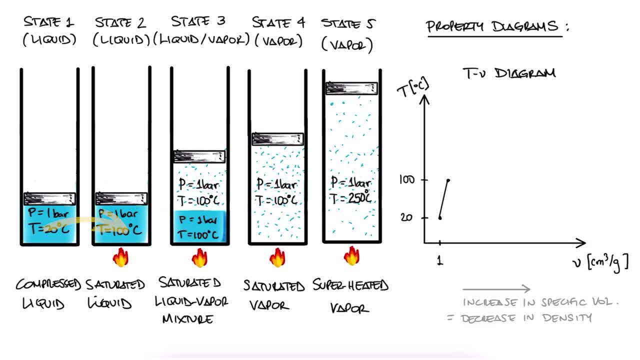 water goes from 20 to 100 degrees Celsius to state 2, then, without going up, and then up or down moves right, meaning the specific volume increases dramatically while water becomes vapor, passing through 3 to state 4.. And finally, we go up to 250 degrees Celsius. 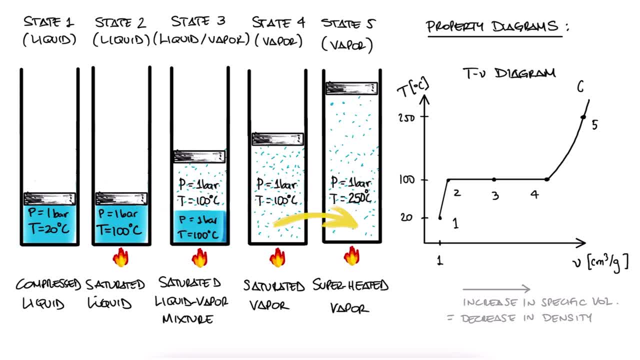 while also increasing the system's specific volume moving right. Remember that all of these changes, due to the fact that we're using a piston-cylinder system, occur at the same pressure, like we explained earlier. With this example, we can look at two definitions. 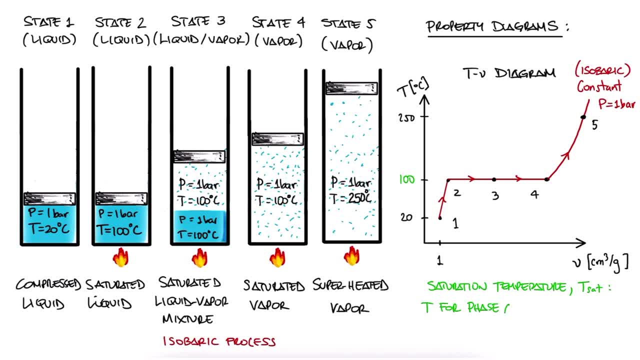 Saturation temperature, T sat, is the temperature at which phase change occurs at constant pressure. On the other hand, we have the saturation pressure P sat, which is the pressure at which phase change occurs at constant temperature. This one's harder to grasp and we'll talk. 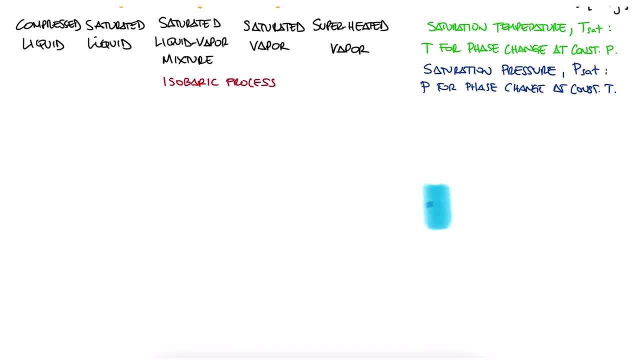 a lot more about it in a later lecture, but for now just picture that we have water at a constant temperature, let's say 95 degrees Celsius, and we lower the pressure from one atmosphere to, let's say, 0.8 atmospheres. 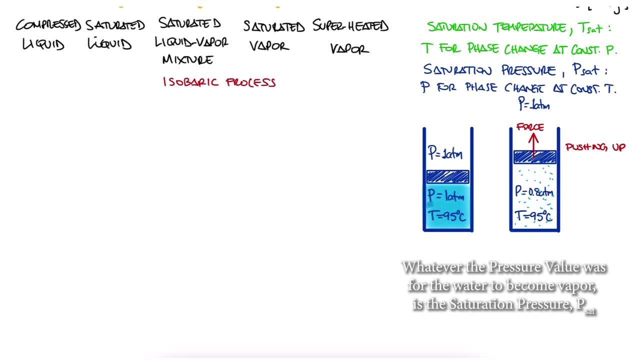 This is exactly what happens when you're in a high altitude location. You're up in the mountains- let's say Denver, Mexico City, Bogota- and you're trying to boil water. Would you have to bring up the temperature to 100 degrees Celsius for it to boil? No, In these. 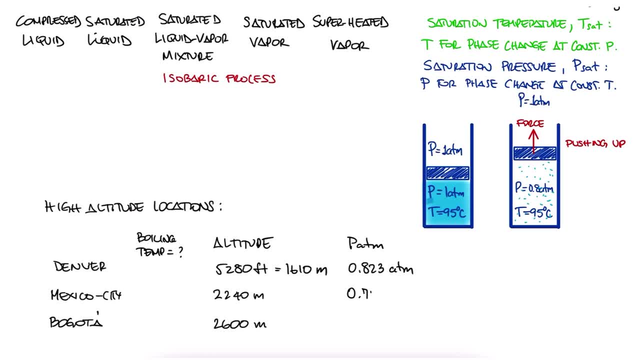 cities and depending on the altitude and therefore the atmospheric pressure there, the boiling temperature can be way lower, like, for example, 90 degrees Celsius in Bogota County, And the same is true for high pressure. A pressure cooker is nothing more than a pot. 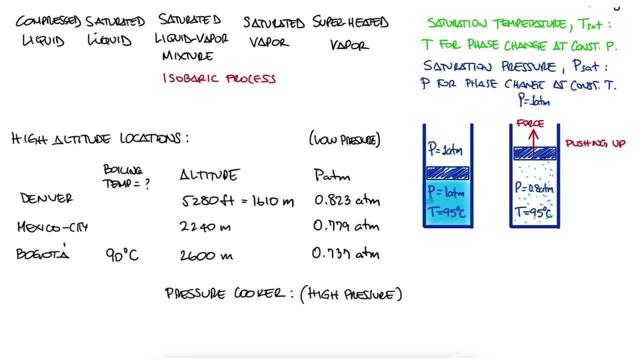 that can have a pressure higher than that of the outside atmospheric pressure. So if your pressure cooker is set to 15 psi- and, by the way, that's gauge pressure, which means that the absolute pressure is roughly 30 psi- water can still be liquid at 121 degrees Celsius. 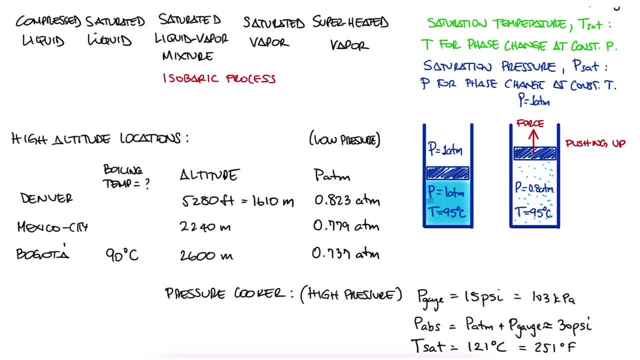 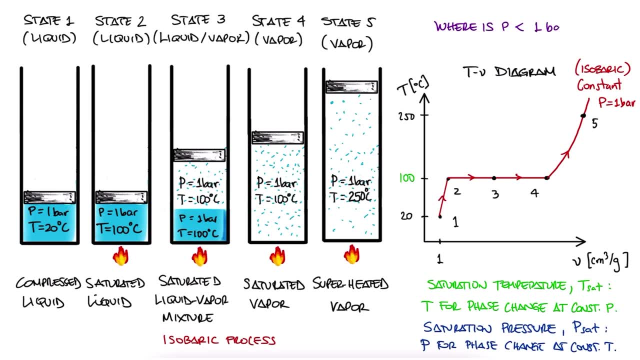 which of course results in food cooking much quicker- the entire purpose of using a pressure cooker. So, going back to our T-V diagram, if pressure is not 1 atmosphere, but lower or higher, what changes? Well, we know that at lower pressure values- high elevation cities, for example- 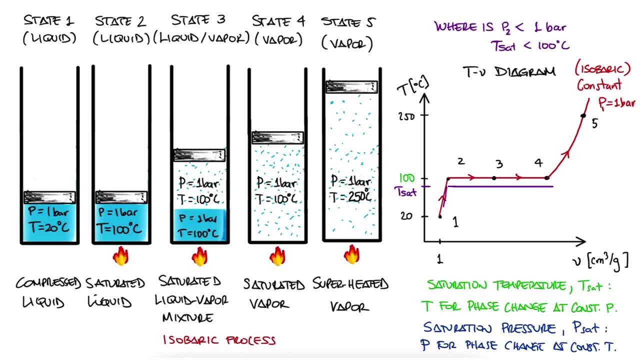 the boiling temperature is also lower and this affects the temperatures lower and higher than the boiling temperature. And the opposite is true. for higher pressure values In a pressure cooker, the temperature needed to boil water is higher and again this affects volumes below and above boiling. 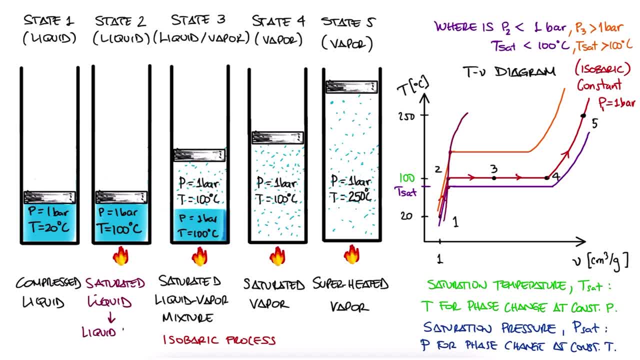 temperature. If we join all saturated liquid points on the left and all saturated vapor points on the right, we obtain the saturation dome. Everything inside the dome is saturated liquid vapor, everything to the left of the dome is compressed liquid and everything to the right of the dome is superheated vapor. 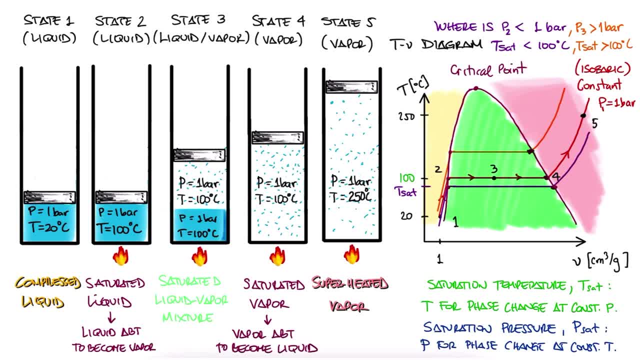 The top of the dome is called the critical point, where anything above it is a supercritical fluid, a fluid that has properties of both liquids and gases. but none of that will be of interest in a Thermo 1 course. The data for every single state of water is found in textbook tables where properties 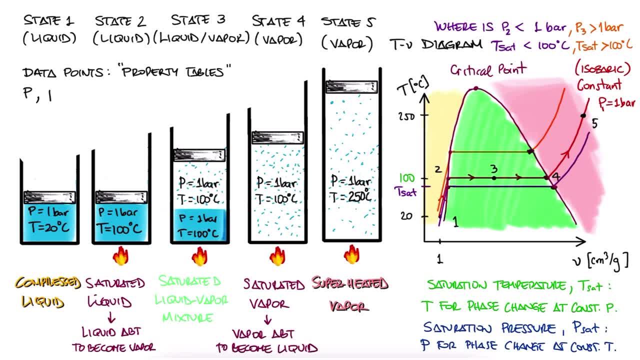 are tabulated for different values of pressure, temperature, specific volume, specific internal energy, specific enthalpy and specific entropy. We'll get to what those last two mean in a later lecture link below. We call these property tables and you can find tables like these for substances other. 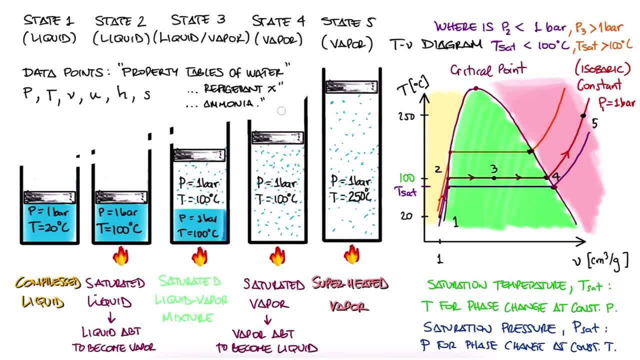 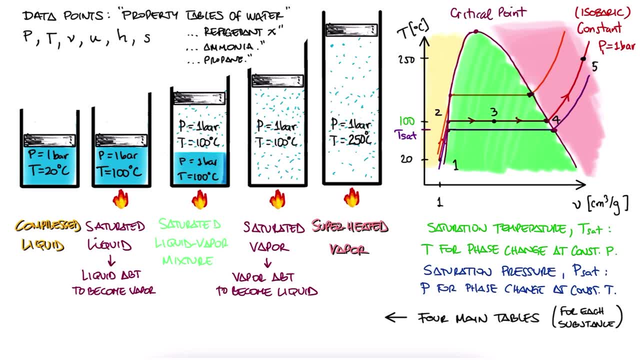 than water, for example, refrigerants or coolants. The specific table you use will depend on the region your substance is located: One table for compressed liquid, one table for superheated vapor and two for saturated liquid vapor. One if you're looking up pressure first and another one if you're looking up temperature. 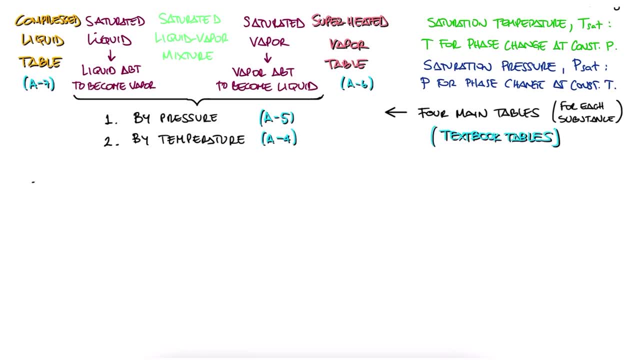 first With these tables. if we have any two of these properties, as long as they are independent, we can find the remaining values from this list for that specific table. Thank you for watching. For example, if we have temperature and specific volume of water specifically, we can find. 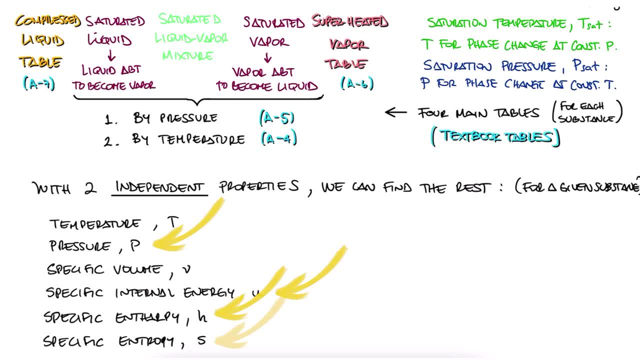 the pressure, the specific internal energy, enthalpy and entropy. Now, independent properties are any combination of these that are not pressure and temperature. We'll learn more about why that is later. To briefly explain it here: think about this. 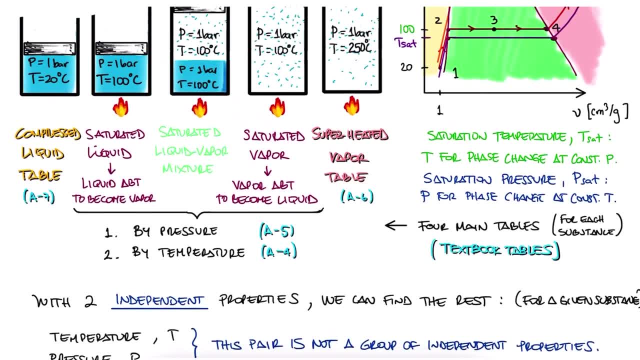 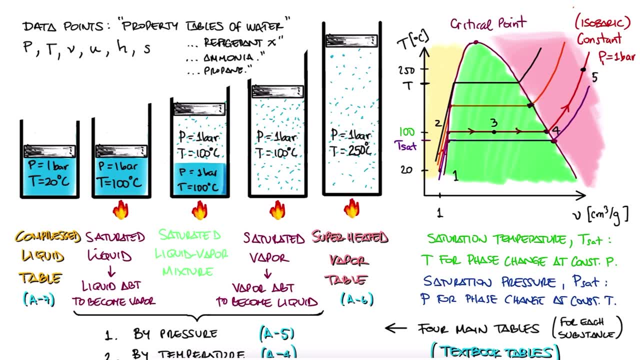 If we know the pressure and the temperature, can we always find the specific volume of our substance? The answer is no. For a given pressure, meaning any one of these lines, it might be that the substance is in the saturated liquid vapor region and therefore the specific volume can be anything that lies. 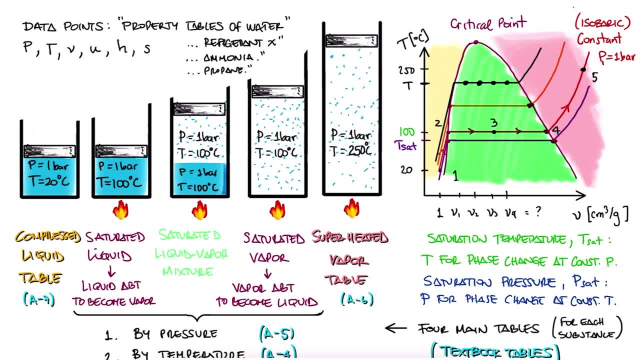 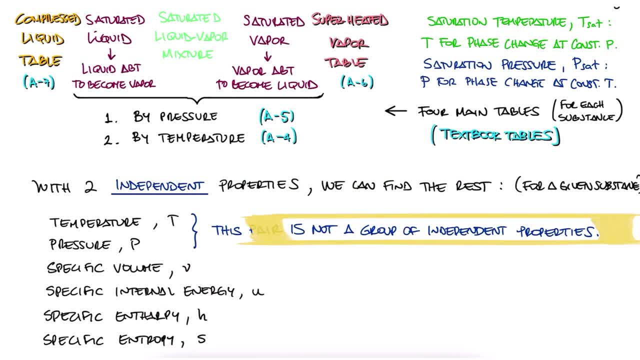 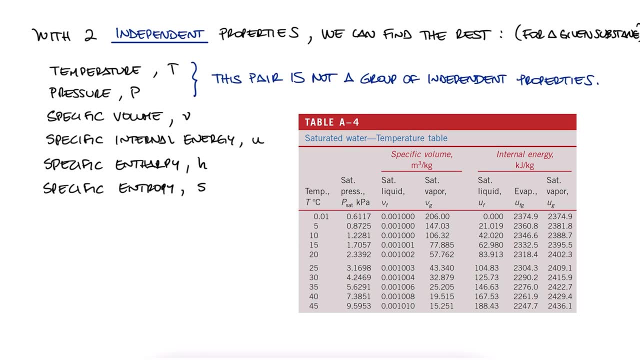 on that horizontal line. Sometimes it might be enough, but sometimes it isn't so. that's why we call the combination of pressure and temperature a not-independent properties combination. Now, what if your exact number for temperature is not in the table? What if the table shows property values for 30 and 35 degrees Celsius? 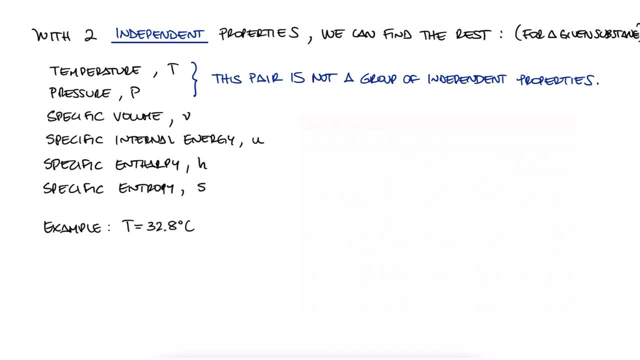 Well, what we normally do in thermodynamics is interpolate, and a big, big part of thermo problems is tabulating these values. However, and listen closely to this, even though this is the typical approach in any thermo course, any school, any textbook, and it is indeed usually enough for solving thermo, 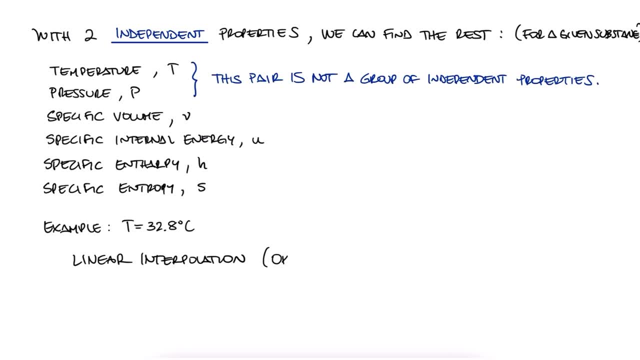 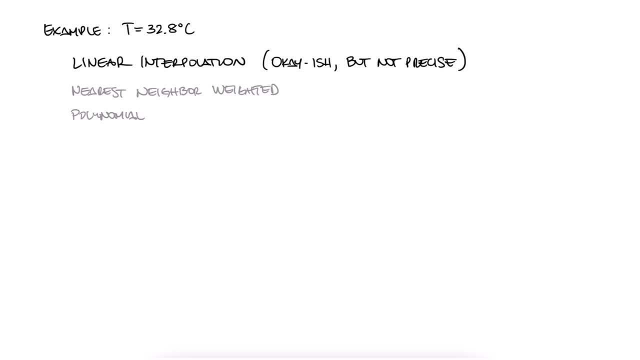 designs. this oversimplified linear interpolation is not precise. If you've already taken a course like numerical analysis before, you know that there are multiple ways of getting much more accurate values when interpolating In general. you can still use the property tables for steam and coolants in your thermo. 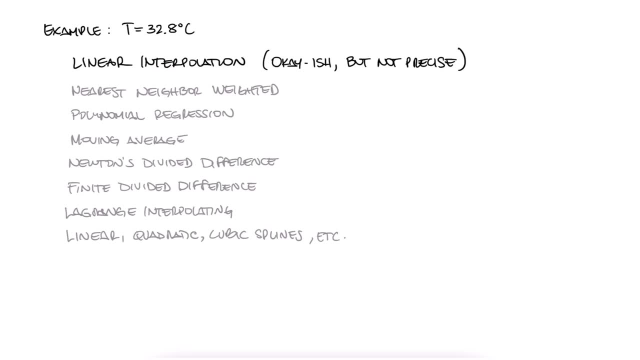 textbook and we will be going over simple linear interpolation in the next lecture linked below, specifically for explaining how we do interpolation for these values. But an easier and much quicker alternative to find properties is to use online tools or software like EES, where you enter two property values like internal energy and temperature, and 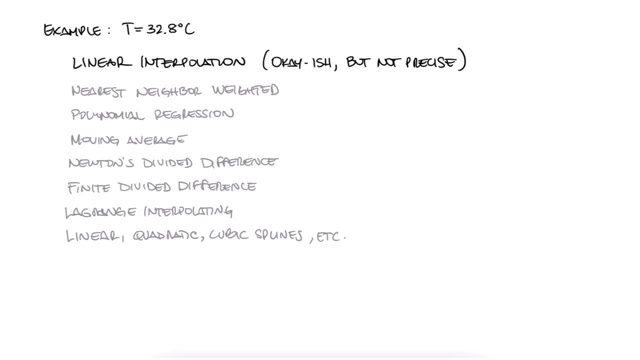 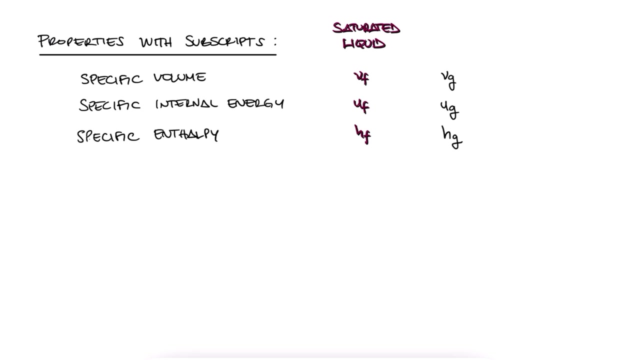 you get all of the properties as output, no time wasted on interpolating and lower inaccuracies than linear interpolation. Now, specific volume, internal energy, enthalpy and entropy can have subscripts. These can be F for saturated liquid, G for saturated vapor or Fg for the difference. 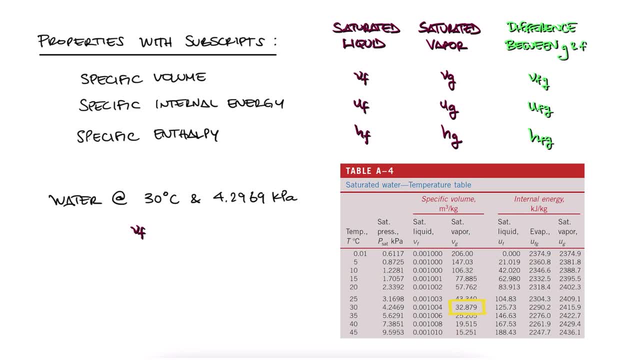 between the two. For example, Vg is the specific volume for a saturated vapor and Vg is the difference between the two. Vf is the specific volume for a saturated liquid and if you ever get Vfg, it just means the difference between the two. 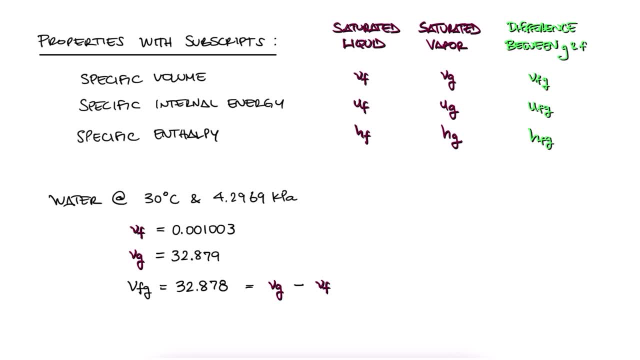 Which is sometimes useful if you're trying to find a change in specific volume, although more useful for energy enthalpy and entropy for a substance that went from saturated liquid to saturated vapor, Since there's four main tables, if you're going to use the tables to find the properties. 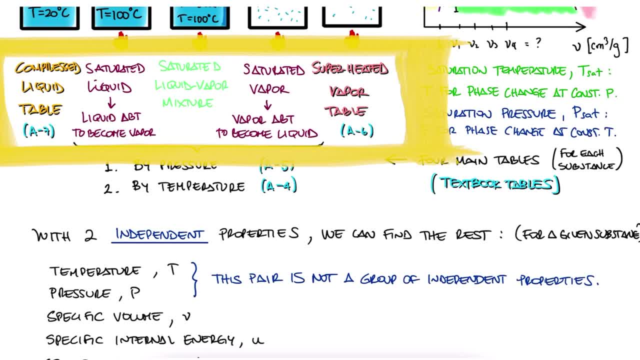 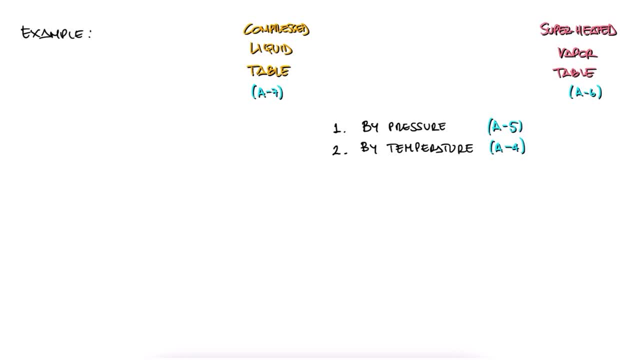 that you're looking for. you first need to identify the state or region of your substance: Saturated, compressed or superheated. Let's try identifying that with a simple example. that covers everything we learned today, and if you want to see more complex examples on this same topic, make sure to check out the 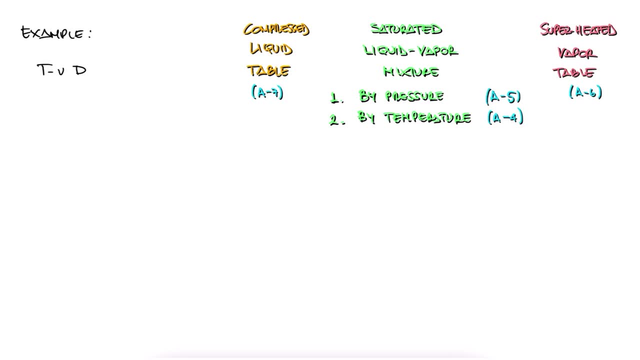 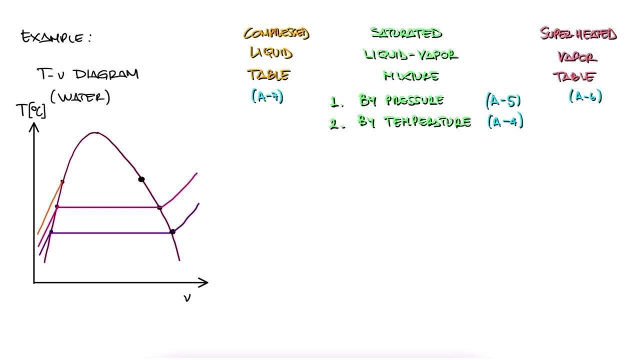 example links in the description below. Let's say we are drawing a TV diagram for water and we want to find the coordinates for these six points for three pressure situations for water: 100, 300, and 618.23 kilopascals. 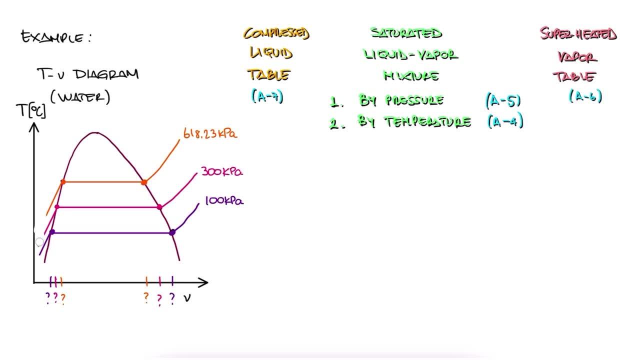 Since these points are the same, we can use the same equation to find the coordinates for these three pressure situations for water. These points are the saturated liquid and saturated vapor values for water Out of the four options I mentioned earlier. it makes sense to look up the tables for saturated 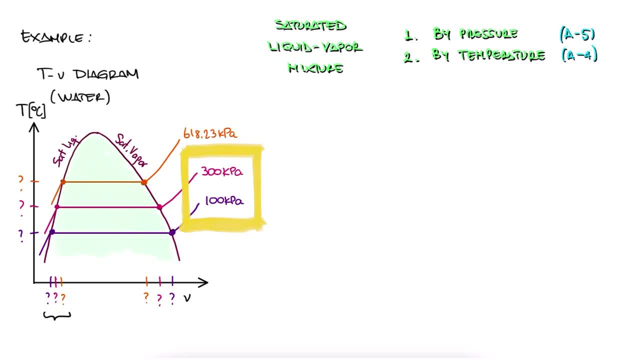 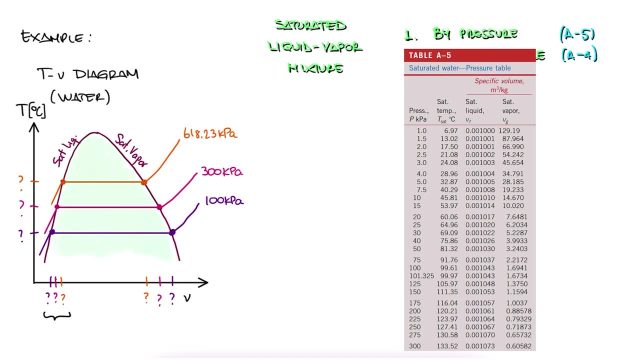 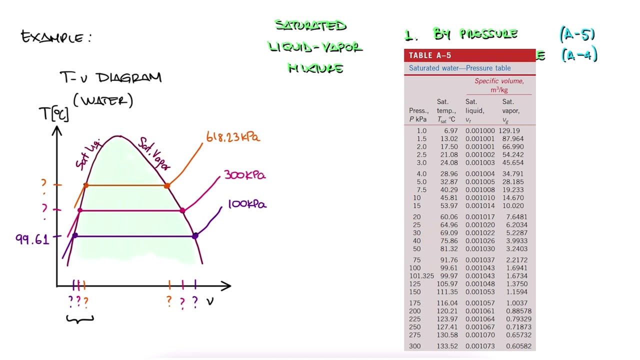 water. For the first two values of pressure, we'll use the saturated pressure table. This means the table for saturated liquid vapor, where vapor is the first column For 100 kilopascals, we see that the saturation temperature is 99.61 degrees Celsius and 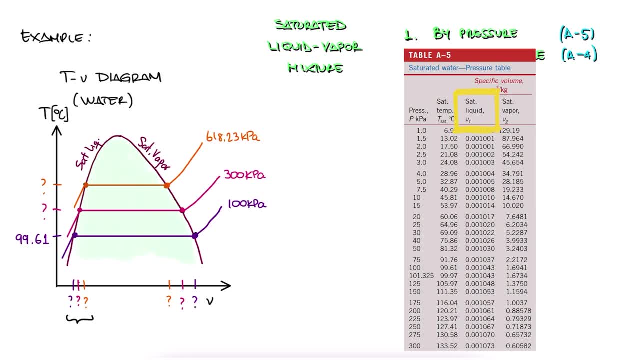 that the saturated liquid has a specific volume Vf of 0.001043 cubic meters per kilogram and that the saturated vapor has a specific volume Vg of 1.6941 cubic meters per kilogram. Looking at 300 kilopascals, we see a saturation temperature of 133.52 degrees Celsius. Vf- peanuts. 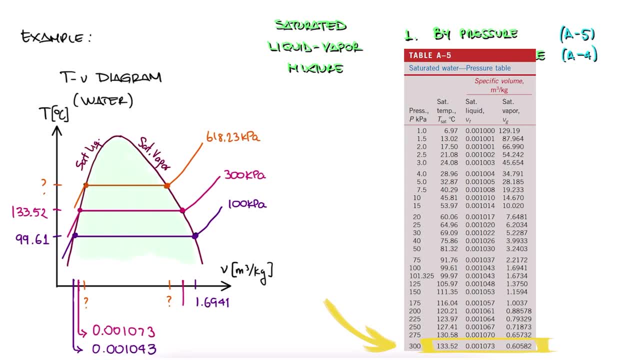 degrees Celsius and 0.01073 degree Celsius. Vf equals 0.001073 and Vg equals 0.60582.. But water is 100 % higher at f 1.. serum, f I water. it known as a mix. 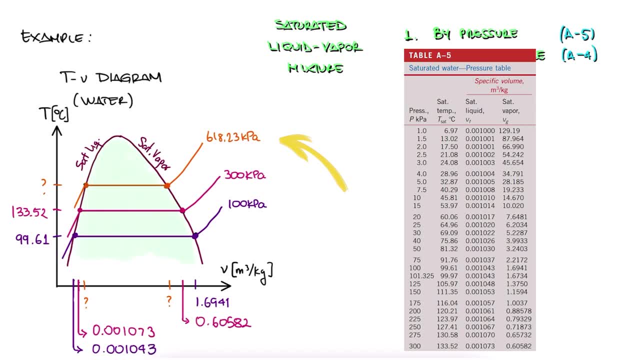 Now, technically, if the third state we want to look for is also given by its pressure, we would use the same table And since the value is not a whole number, we'd have to interpolate. But more often than not these values are given because they correspond to a whole number. for the 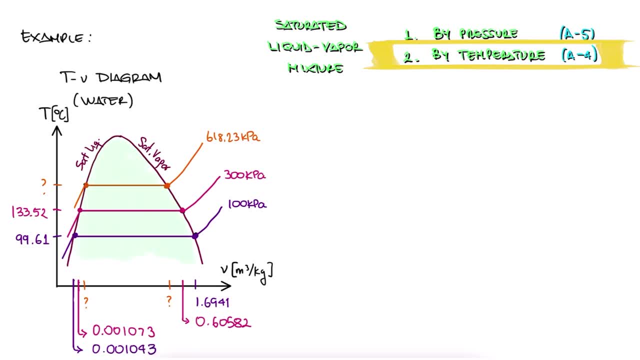 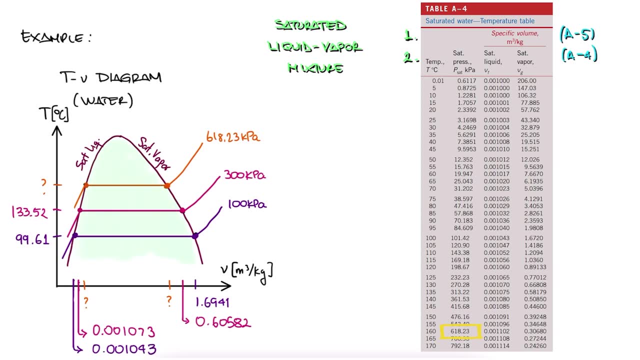 other property, in this case temperature. If we go to the saturated table for temperature, we see that a pressure of 618.23 corresponds to a temperature of 160 degrees Celsius. This is the same as looking up a pressure of 618.23 in the pressure table and finding that. 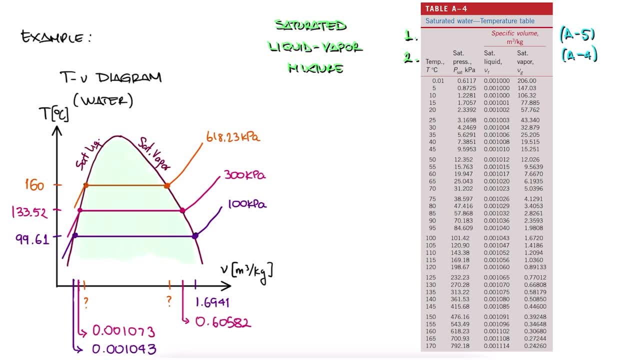 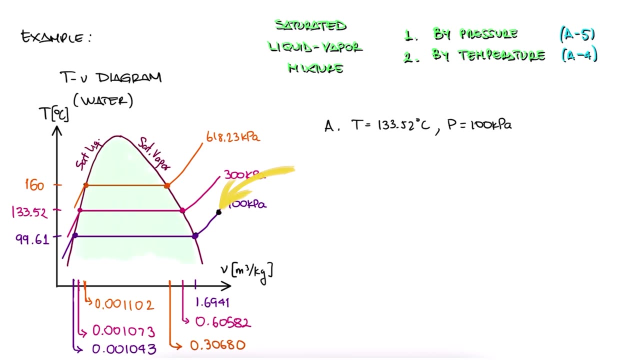 the saturation temperature is 160 degrees Celsius, The specific volumes would be 0.001102 and 0.3068.. And that's it. If, for example, we know that pressure is 100 kilopascals and that the temperature is 133.52 degrees Celsius, what region and table would we use? 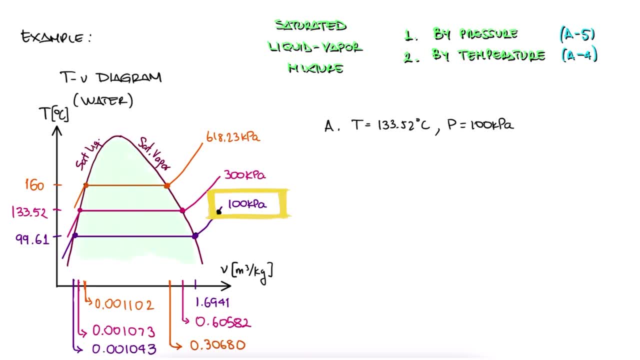 Well, since for 100 kilopascals the saturation temperature is 99.61 degrees Celsius, being at 133.52 means that we are in the superheated vapor region. In this case we'd use the superheated table. What about 300 kilopascals and 133.52 Celsius? 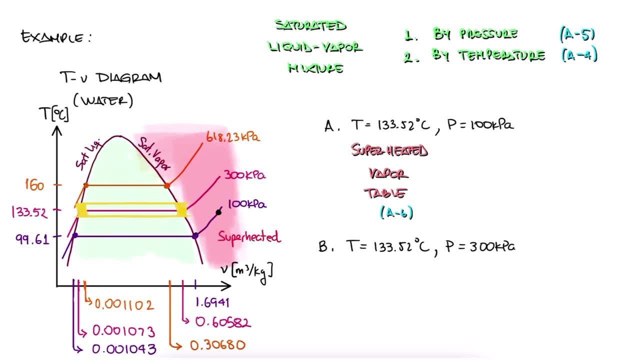 Well, since the saturation temperature is exactly 133.52,, we would therefore use either of the two saturated tables- temperature or pressure. And since the saturation temperature is exactly 133.52,, we would therefore use either of the two saturated tables- temperature or pressure. 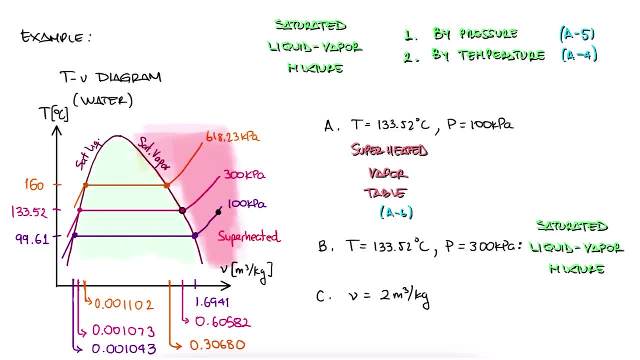 What if we know our specific volume is 2 cubic meters per kilogram and that the pressure is 300 kilopascals? In this case, since the specific volume is higher than that for saturated vapor Vg, we know we're in the superheated region. 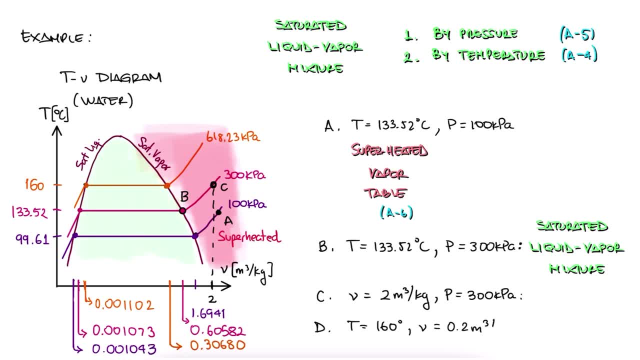 What about 160 degrees Celsius and a specific volume of 0.2 cubic meters per kilogram? Easy, the saturated region. And finally, what can we say about the pressure if the temperature is 160 and the specific volume 0.2??